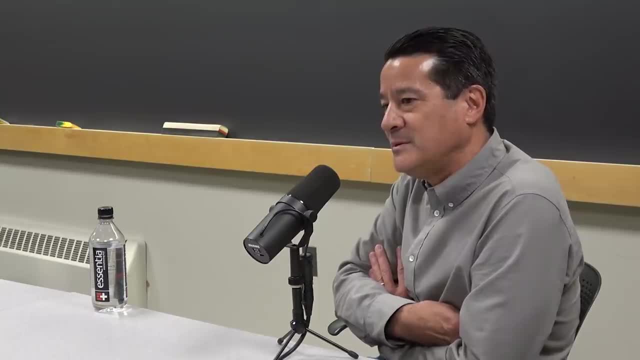 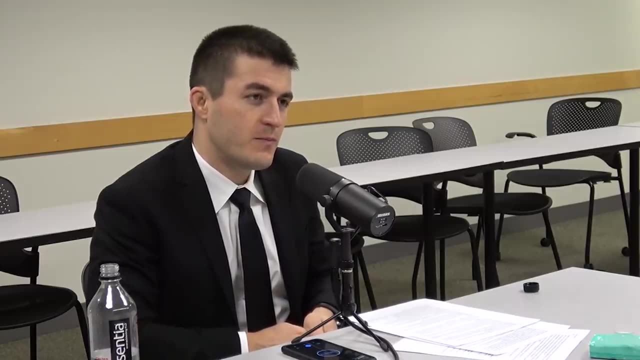 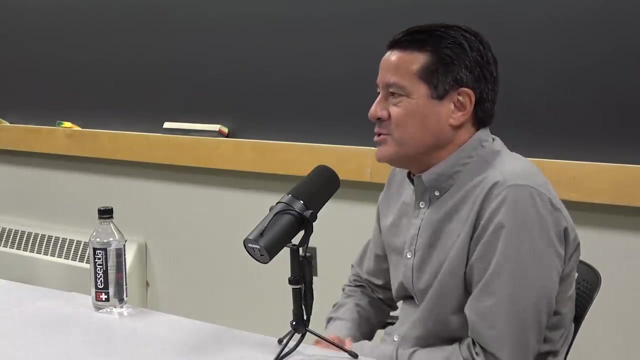 what will happen in the design of platforms? What, to you, is the most beautiful idea that you've encountered in game theory? There's a lot of them. I'm a big fan of the field. I mean, you know, I mean technical answers to that, of course, would include: 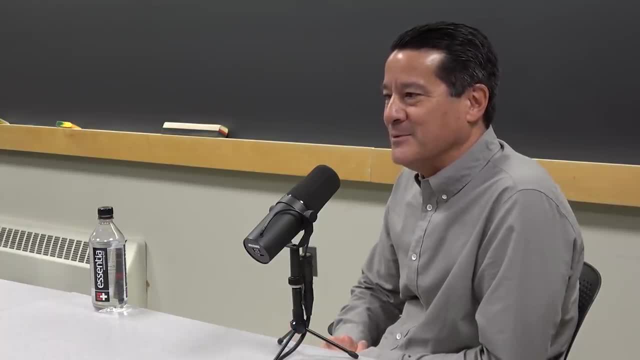 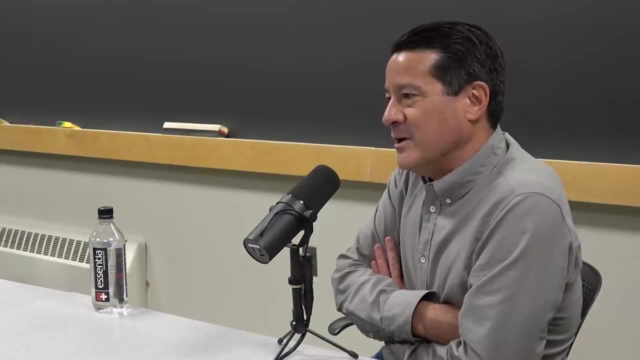 Nash's work, just establishing that. you know, there there's a competitive equilibrium under very, very general circumstances, which in many ways kind of put the field on a firm conceptual footing, because if you don't have equilibrium it's kind of hard to ever reason. 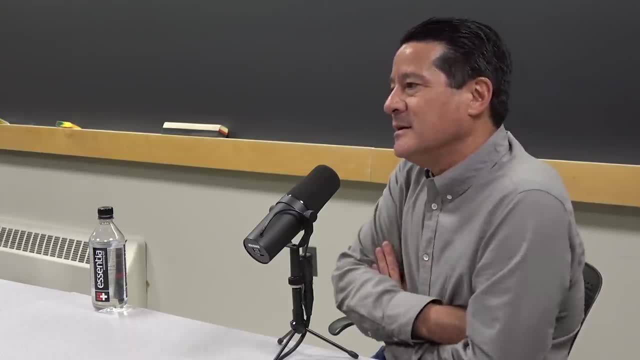 about what might happen, since you're in the game- And I think that's one of the things that I'm really proud of- is just that you can imagine what would happen, since you know there's just no stability. So just the idea that stability can emerge when there's multiple people doing stuff. 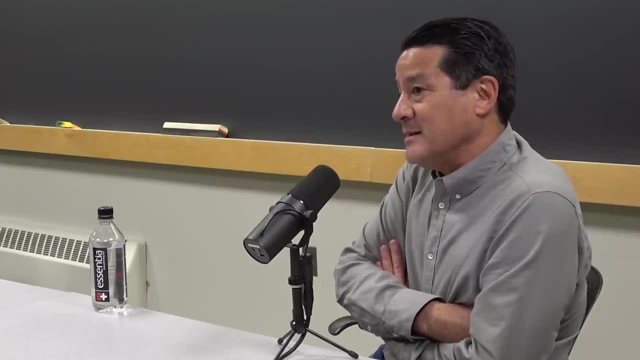 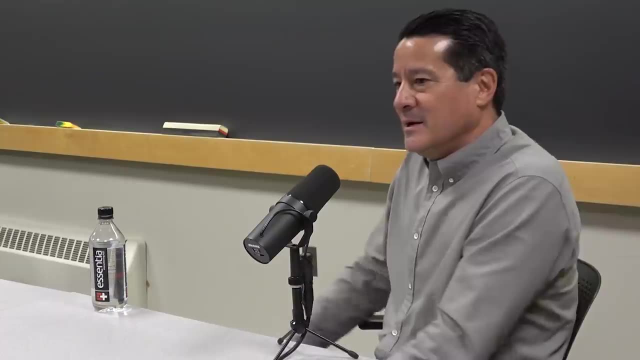 Not that it will necessarily emerge, just that it's possible, right? I mean, like the existence of equilibrium doesn't mean that sort of natural iterative behavior will necessarily lead to it In the real world. Yeah, Maybe answering slightly less personally than you asked the question. 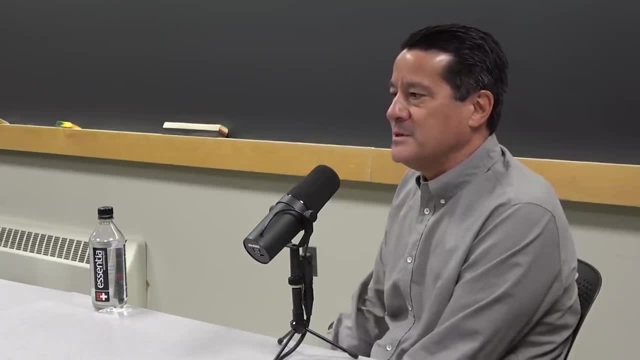 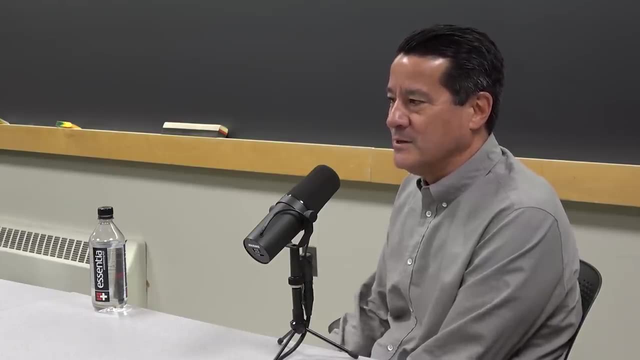 I think within the field of algorithmic game theory, perhaps the single most important kind of technical contribution that's been made is the realization between close connections between machine learning and game theory and in particular between game theory and the branch of machine learning that's known as no regret learning, And this sort of provides. 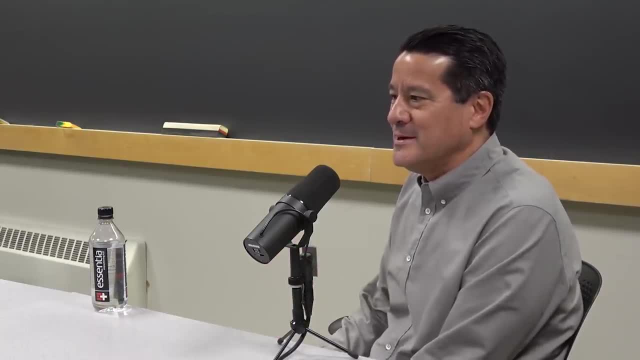 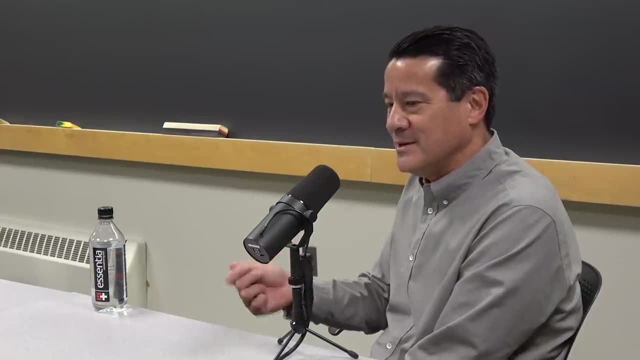 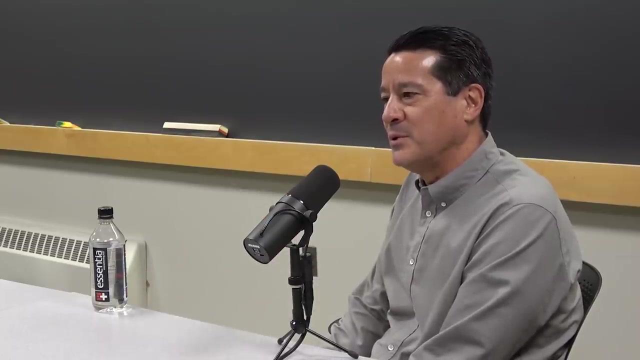 a very general framework in which a bunch of players interacting in a game or a system, each one kind of doing something that's in their self-interest, will actually kind of reach an equilibrium, and actually reach an equilibrium in a pretty you know, a rather you know. 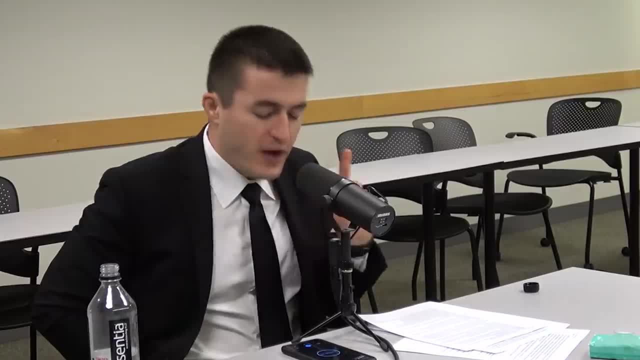 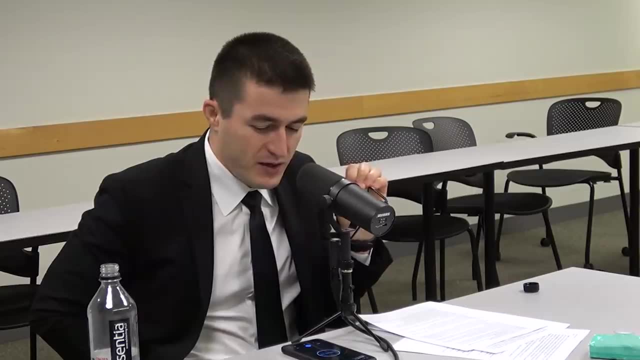 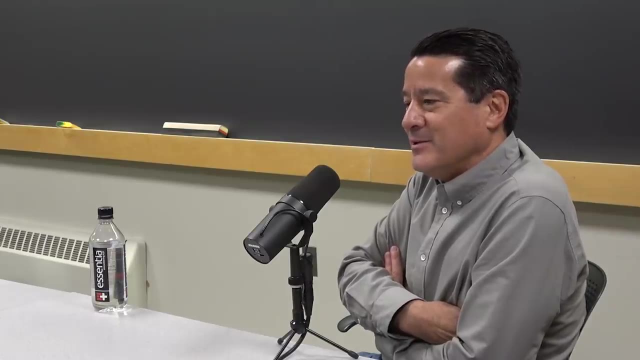 short amount of steps. So you kind of mentioned acting greedily can somehow end up pretty good for everybody, Or pretty bad, Or pretty bad. It will end up stable, Yeah right. And you know, stability or equilibrium by itself is not necessarily. 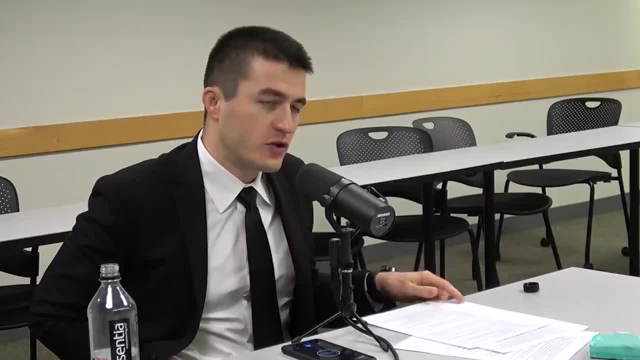 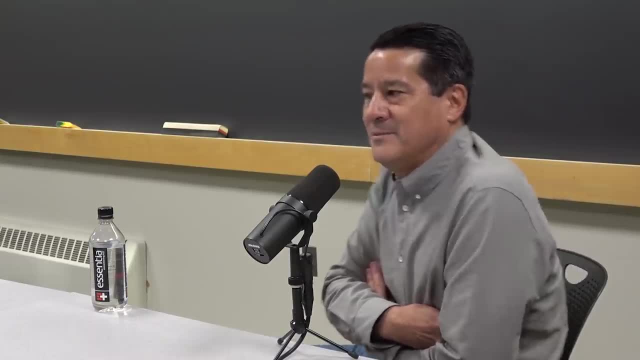 either a good thing or a bad thing. So what's the connection between machine learning and the ideas? Well, I mean, I think we kind of talked about these ideas already in kind of a non-technical way, which is maybe the more interesting way of understanding them first, which is, you know, 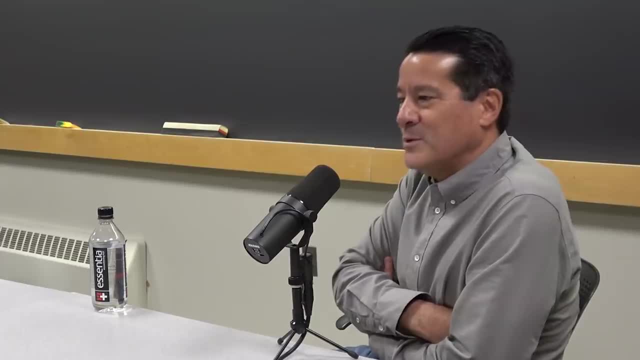 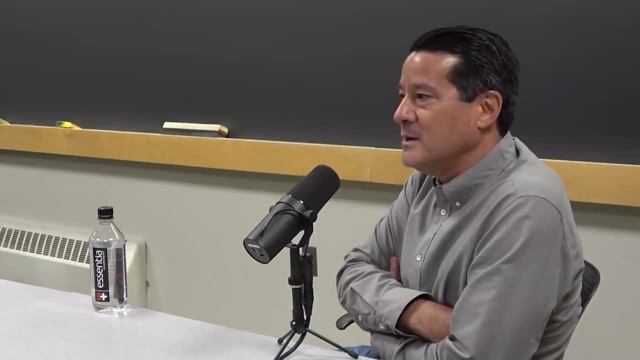 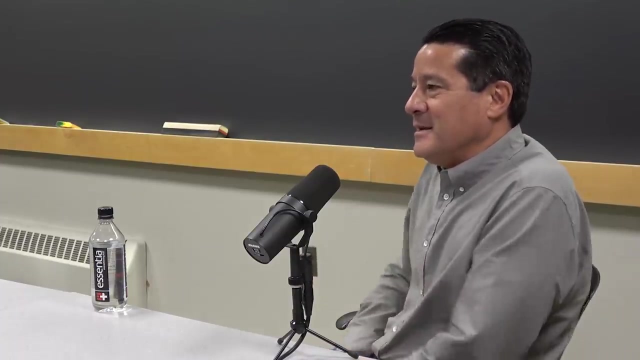 we have many systems, platforms and apps these days that work really hard to use our data and the data of everybody else on the platform to selfishly optimize on behalf of each, each user. Okay, So you know, let me, let me give, I think, the cleanest example. 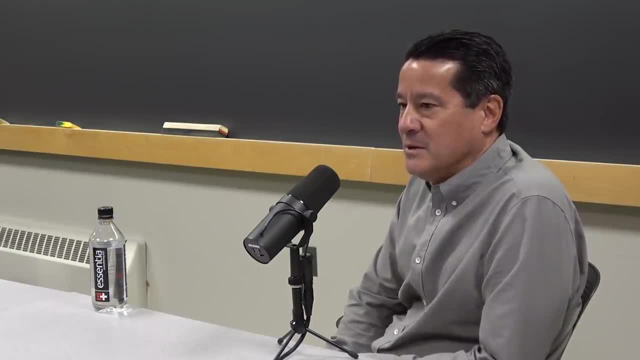 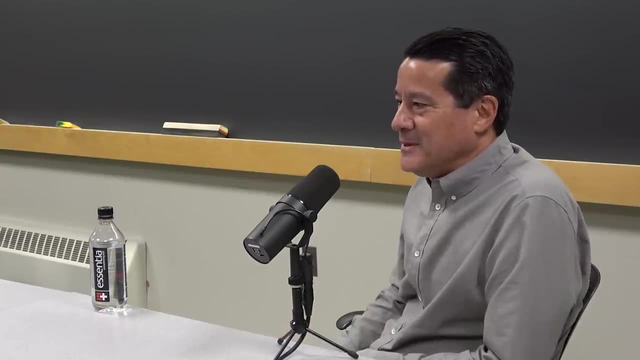 which is just driving apps, navigation apps, like you know, Google Maps and Waze, where you know miraculously- compared to when I was growing up, at least you know the objective would be the same when you wanted to drive from point A to point B. 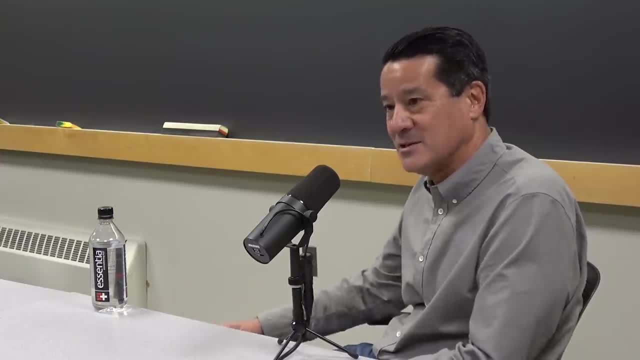 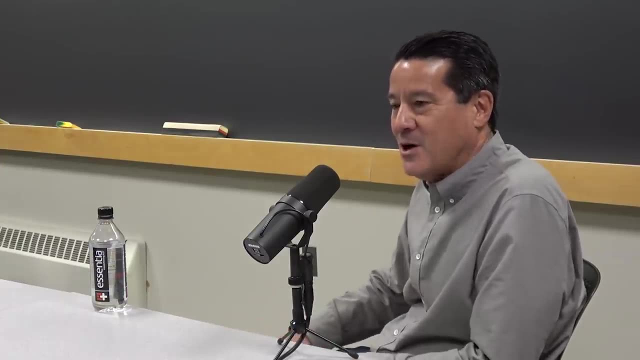 spend the least time driving. not necessarily minimize the distance, but minimize the time right. And when I was growing up, like the only resources you had to do that were like maps in Excel which literally just told you what roads were available, And then you might have like 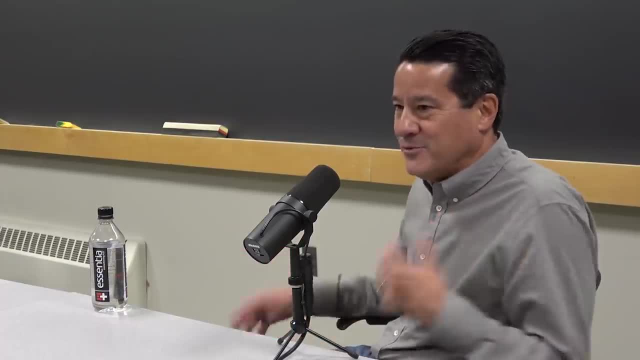 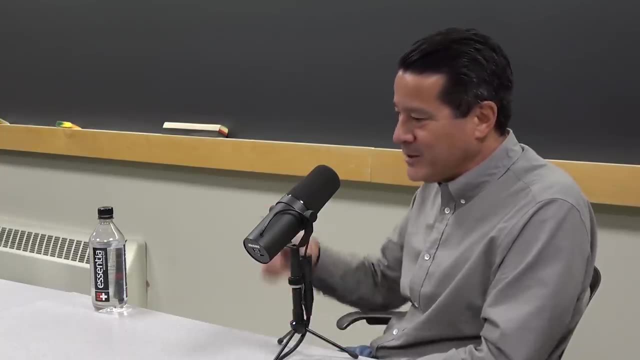 half-hourly traffic reports just about the major freeways but not about side roads. So you were pretty much on your own. And now we've got these apps. you pull it out and you say: I want to go from point A to point B And in response kind of to what everybody else is doing, if you like what. 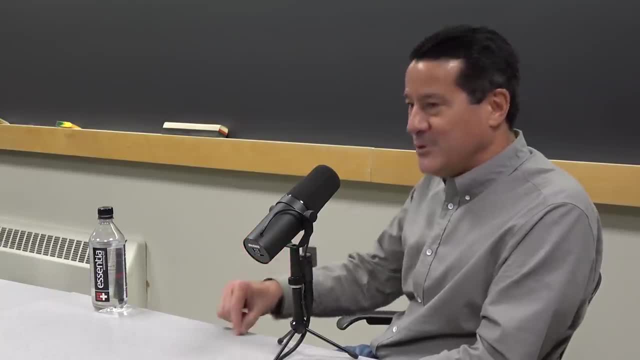 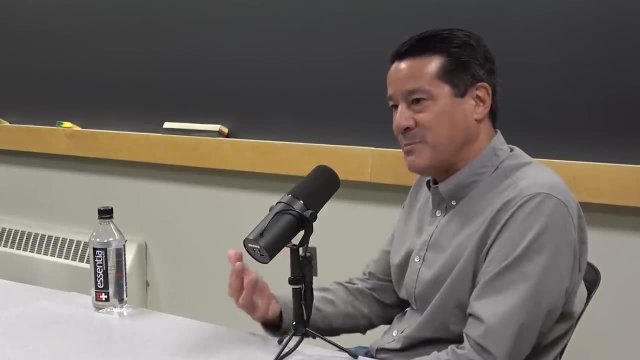 all the other players in this game are doing right now. here's the, the. you know the, the route that minimizes your driving time. So it is really Kind of computing a selfish best response for each of us in response to what all of the rest. 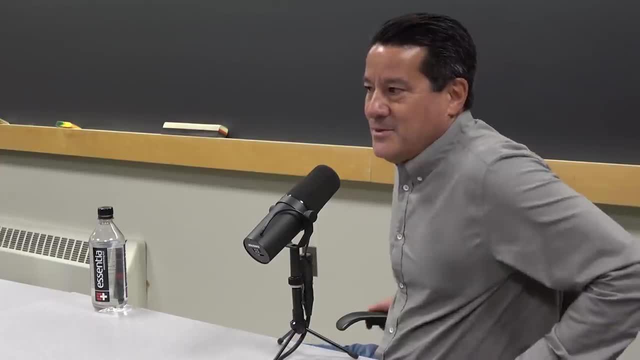 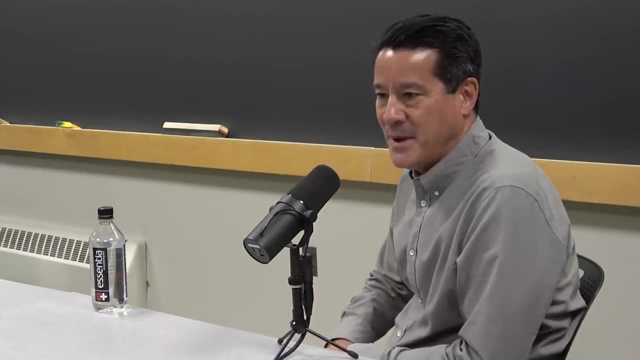 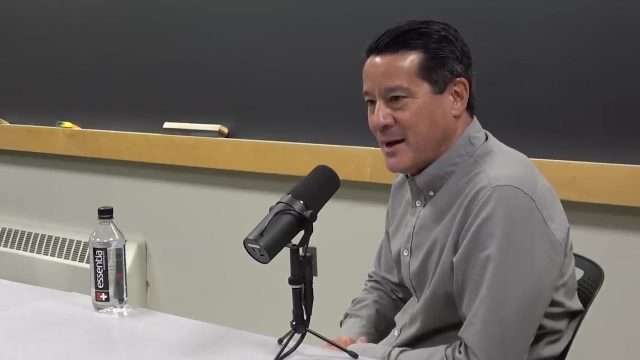 of us are doing at any given moment, And so you know I I think it's quite fair to think of these apps as driving or nudging us all towards the competitive or Nash equilibrium of that game. Now you might ask like well, that sounds great, Why is that a bad thing? Well, you know it's. it's known, both in theory and With some limited studies from actual like traffic data, that all of us being in this competitive equilibrium might cause our collective driving time to be higher, maybe significantly higher than it would be under other solutions.